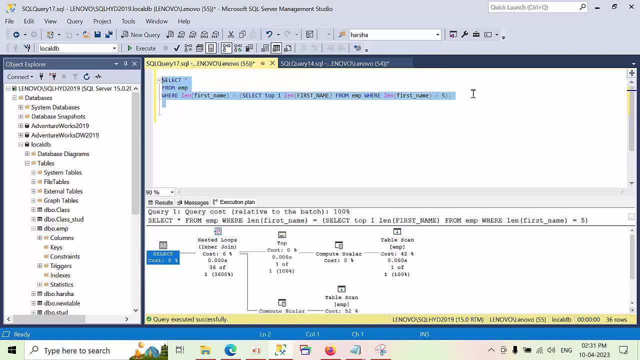 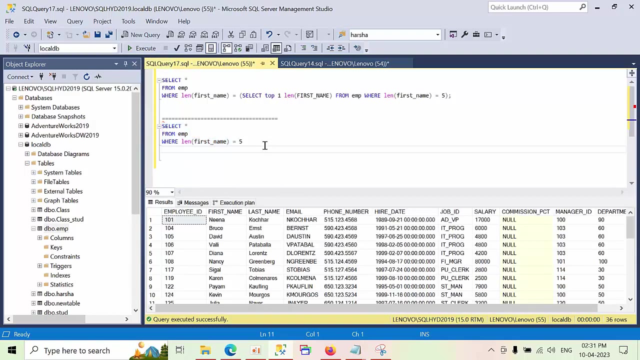 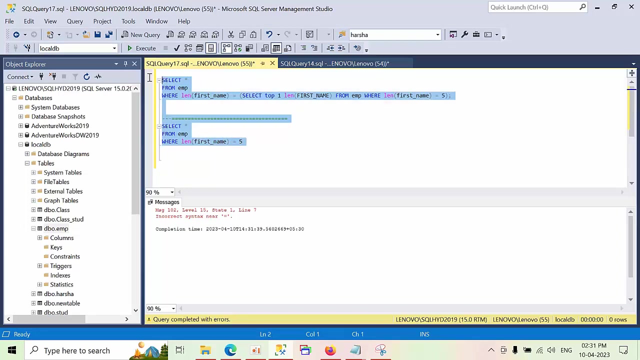 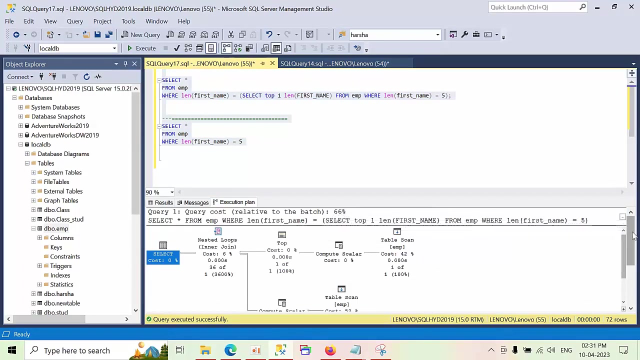 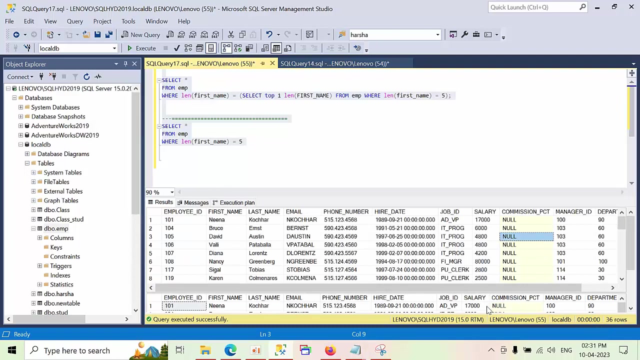 So the query cost and CPU may go high. So sometimes what happened means here we want to think the logic. Okay, so I'm achieving the same. here I'm directly passing five. Okay, so here also I'm having five records. I'm having passing the fire, right, So I, directly I'm giving the hardcoded value. Okay, so I'm. let's see the both execution plans. I need to comment it. See, the query cost is 66%, Now 34%, both. we are seeing 36 records here. 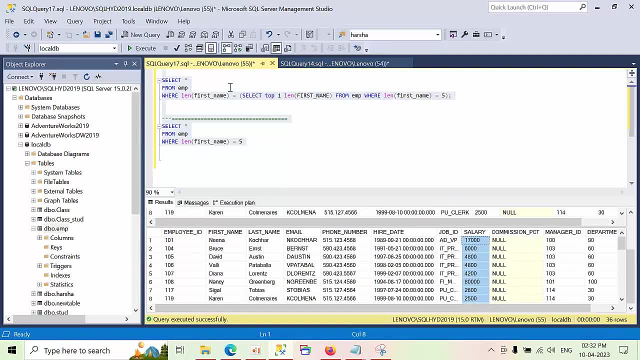 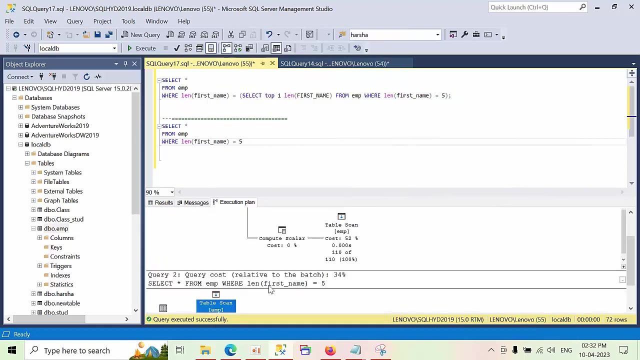 36 records here. So what is the output I am getting here is the same The output I, what I'm getting here, also same. So the same logic. what apply here? the same logic. I have trimmed the query into the simple way. Okay, so if you go here, I'm getting a table scan here. I'm getting a table scan here as well. Okay, but okay, the I mean to say like, if I, let's see how it works. 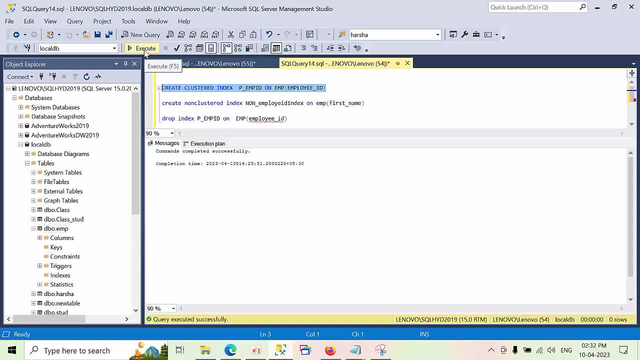 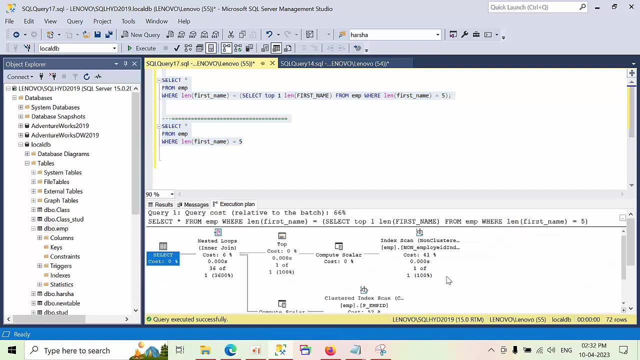 it works in create and clustering on the primary key of employee ID. Okay, I am created a primary key and nonclustered a nonclustered first name, and I am executing this too. again, before it was a table scan, Now it was Index scan, but there is no reduction in the query cost. 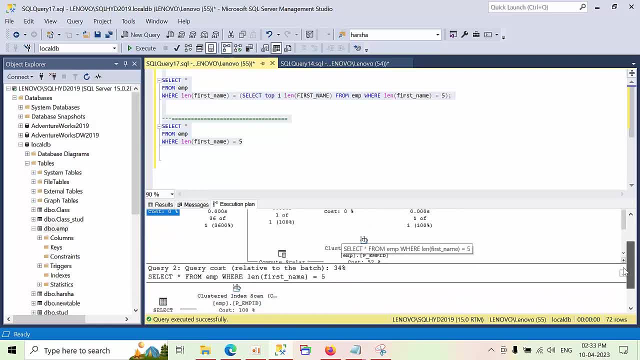 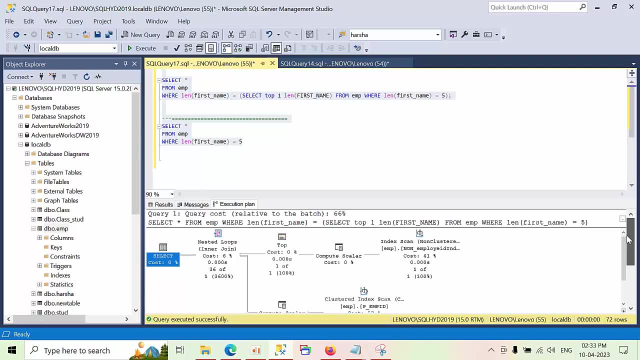 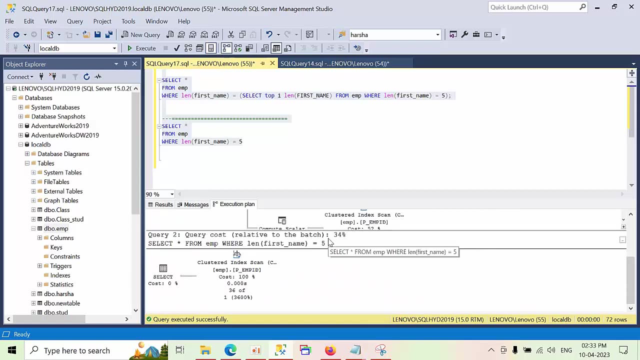 okay, somewhat better, not not so better. okay, we have turned that into integer table scan to index scan. comparing to table scan, index scan is better than the table scan. okay, so now, if you see here, the query cost is 34.. so what i mean to say is, whenever the query is getting a very high or like